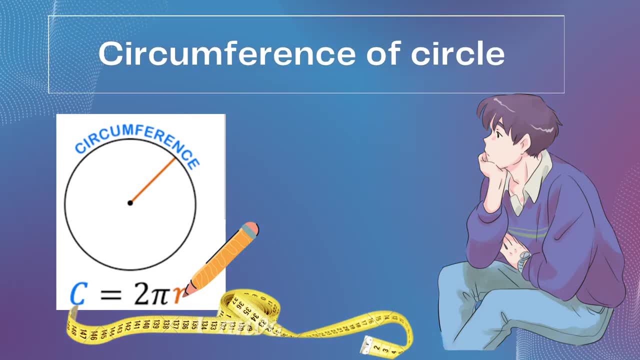 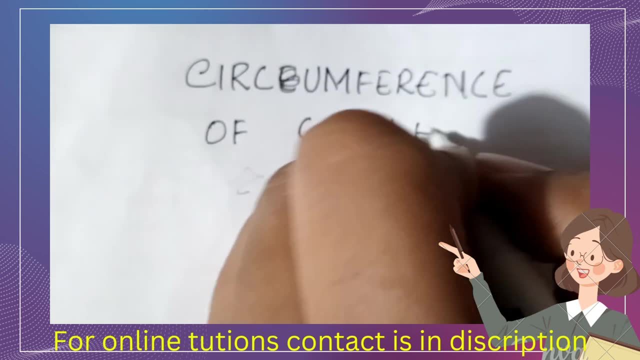 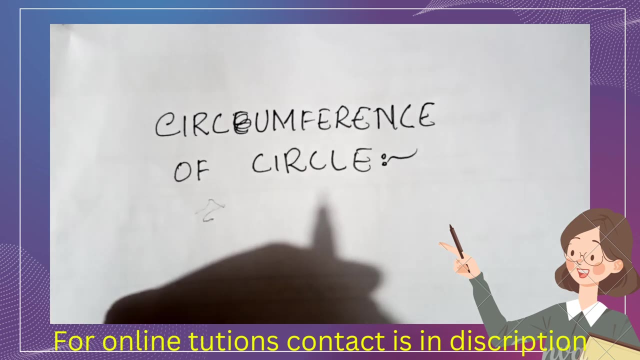 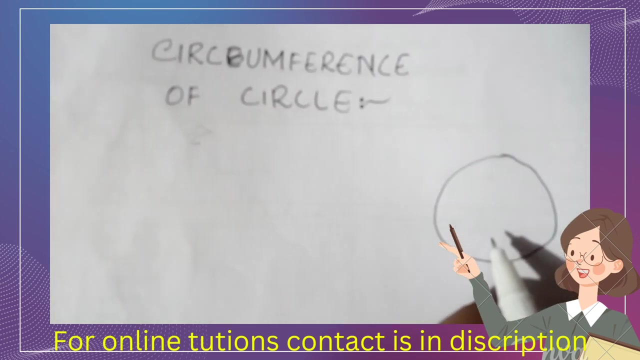 What is circumference of a circle? Here we have discussed in previous video that: what is the circumference of a circle. Now we have a quick review. like a set of a point is called circle. A set of point Equidistance from a center of the circle, This boundary is called. 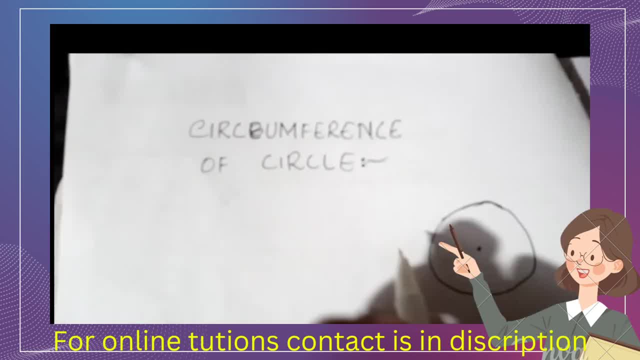 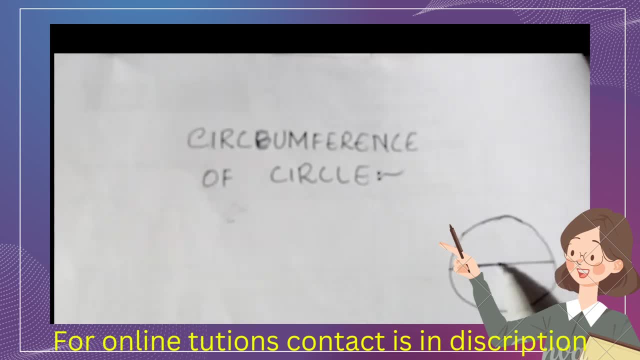 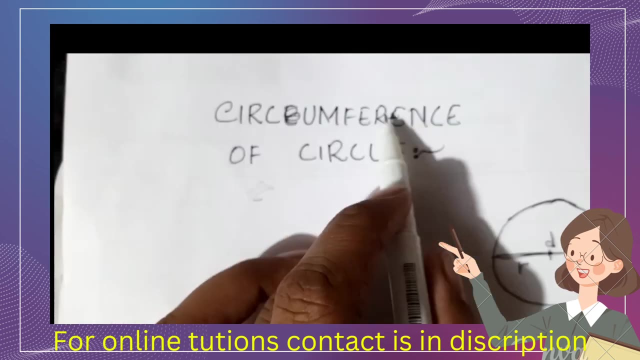 circumference of circle. This is called radius R, denoted by R. The twice of a radius is called diameter. The complete line is called diameter R and R. Now we have two formulas to find circumference of a circle: C. Circumference of a circle is denoted by C. 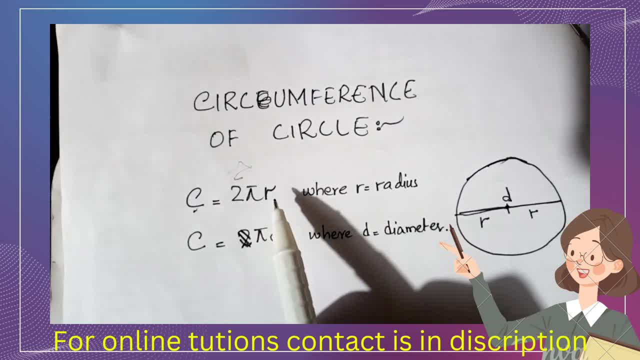 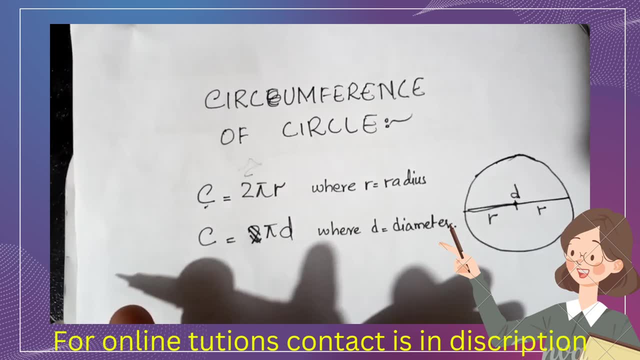 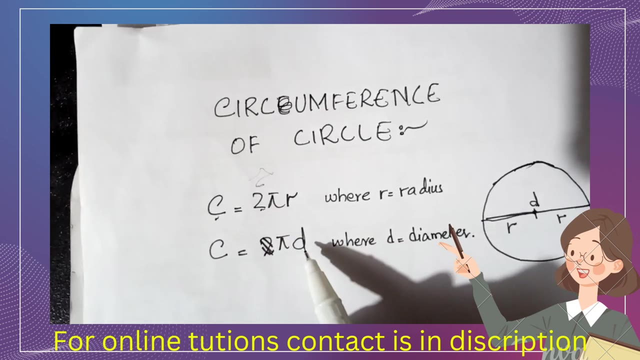 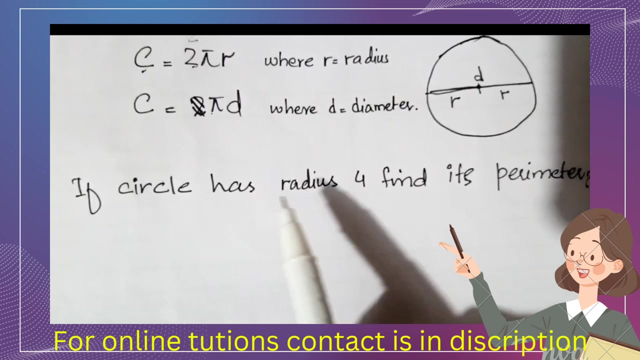 R is the formula to find circumference of a circle. Where R is radius, Pi will be 3.142 or 22 by 7. Diameter is twice of radius. So if we use diameter we use pi d. only Now we have a question: If circle has radius for find its perimeter, Perimeter is also circumference. 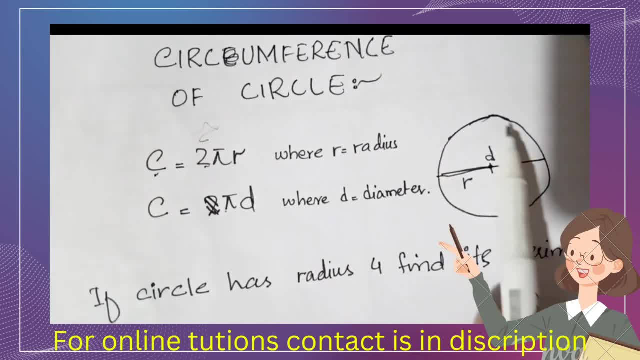 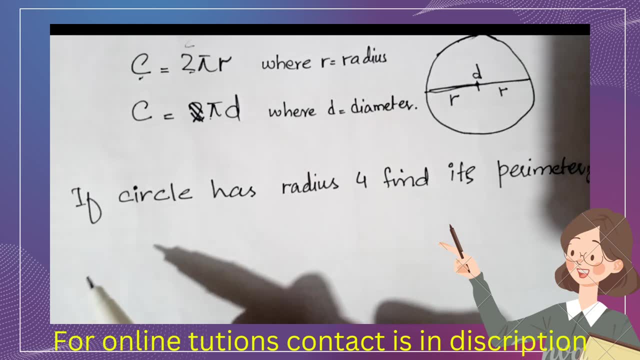 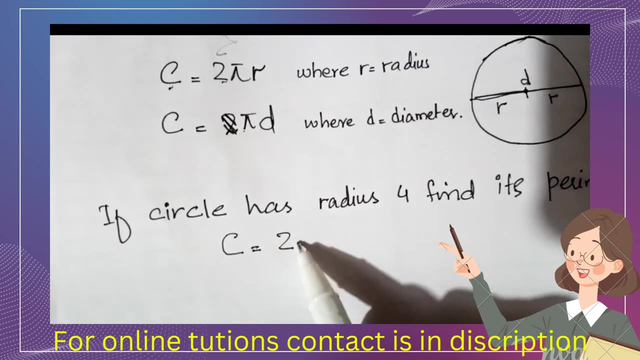 because what is perimeter, Sum of all sides? Here we have only boundary. Then boundary is also called perimeter or circumference of a circle. So here we find circumference of a circle by using formula 2 pi R, because radius is given. C is equals to 2 pi R C. 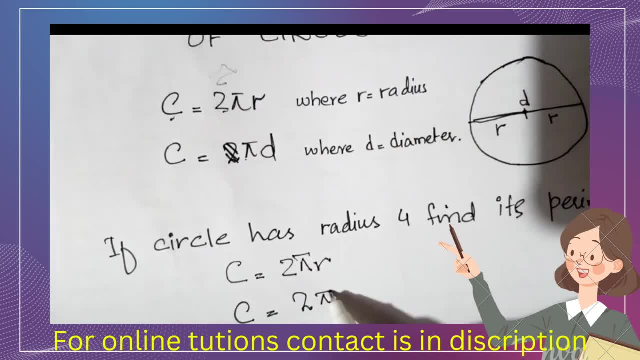 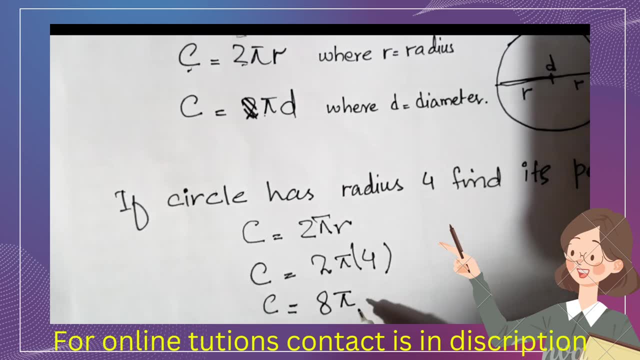 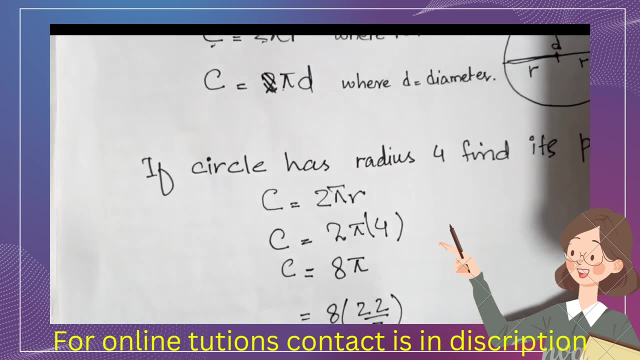 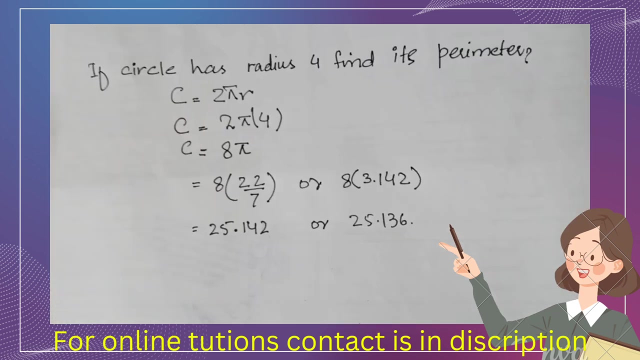 is equals to putting value of radius 2 pi, 4. 4 into 2. 8.. You can leave it here as 8 pi, or you can further multiply it by 8. 22, by 7 or 8. 3.142.. 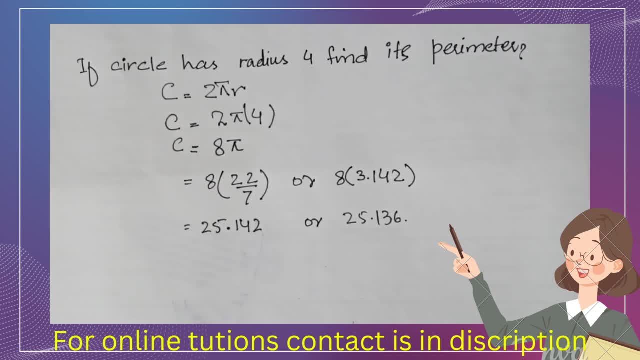 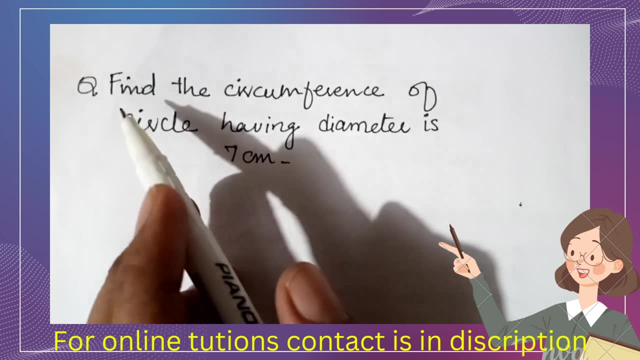 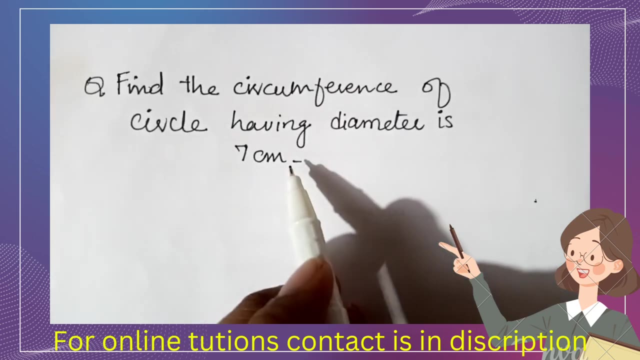 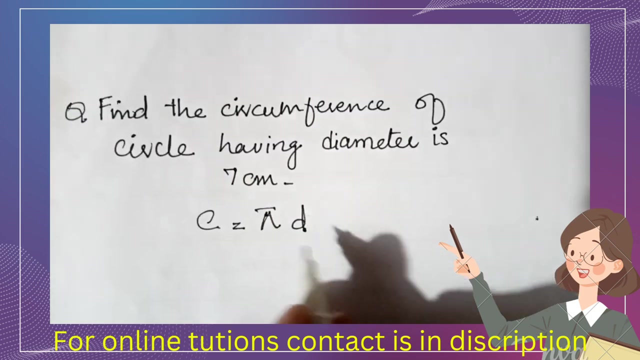 After calculation we get these answers of perimeter of a circle, or we can say circumference of a circle. Now another question: Find the circumference of a circle having diameter is 7 cm. Ok, So we use the formula here is: C is equals to pi, d, d is 7 cm C.